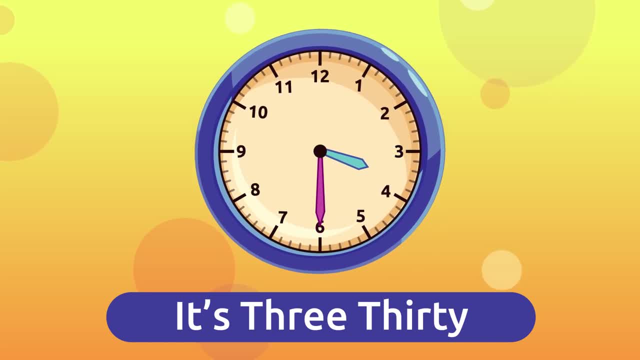 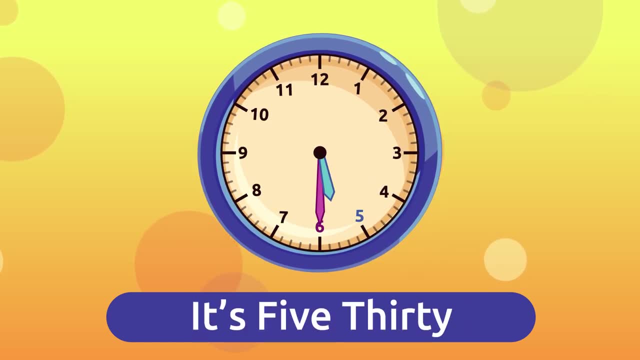 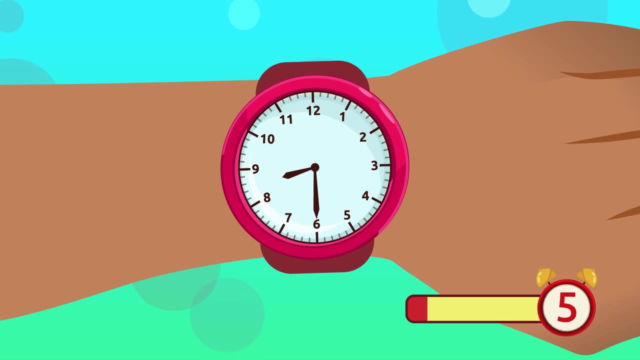 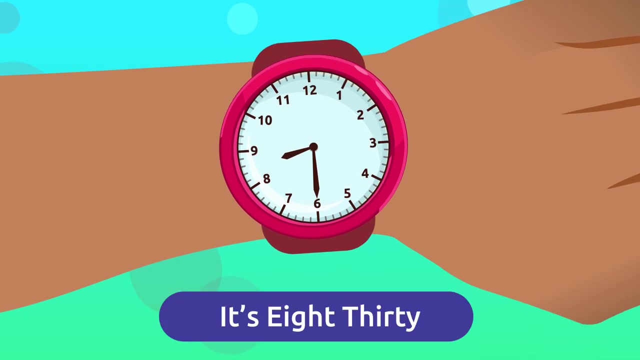 It's 3.30.. It's 4.30.. It's 4.30.. And it's 5.30.. Now it's your turn. What time is it? That's right, It's 8.30.. 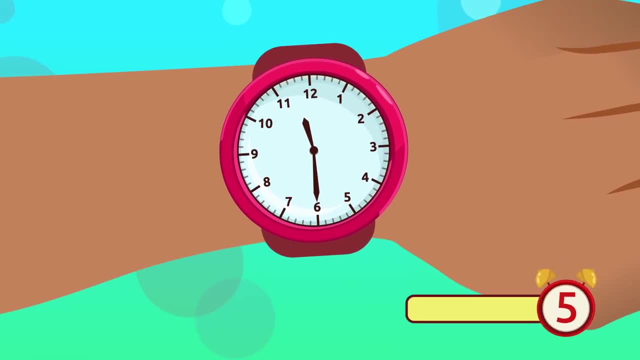 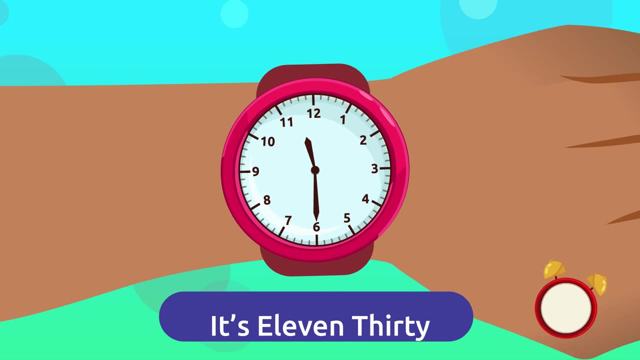 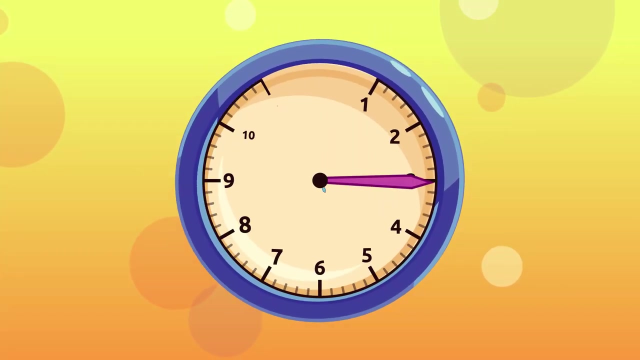 And now, what time is it? That's it, It's 11.30.. When the minute hand is on the 3,, in other words, a quarter of an hour has passed, We say that it is a quarter after the hour. 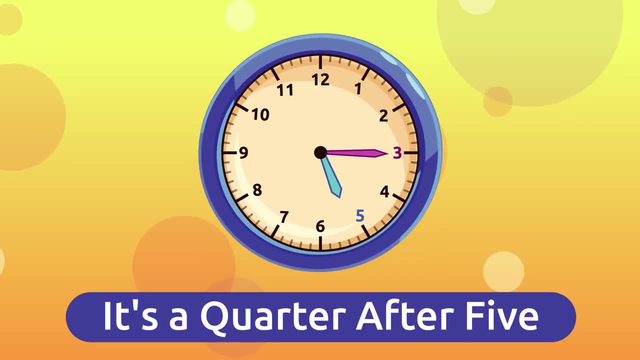 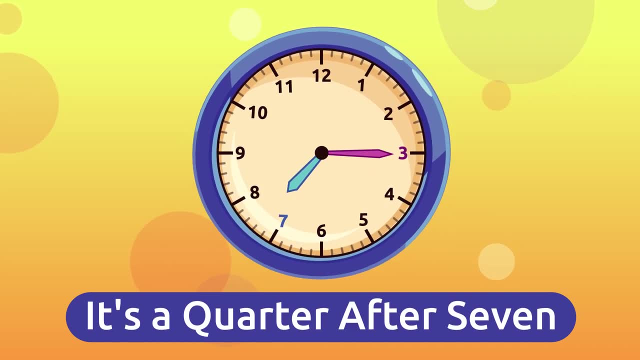 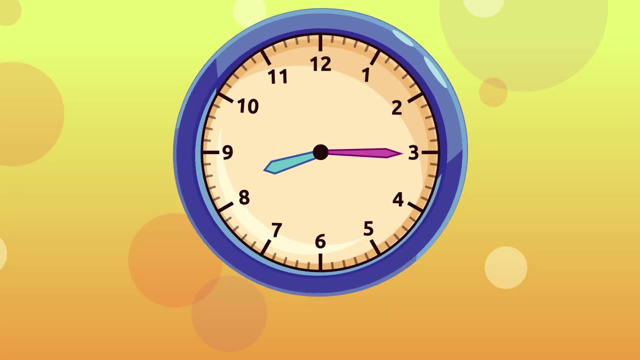 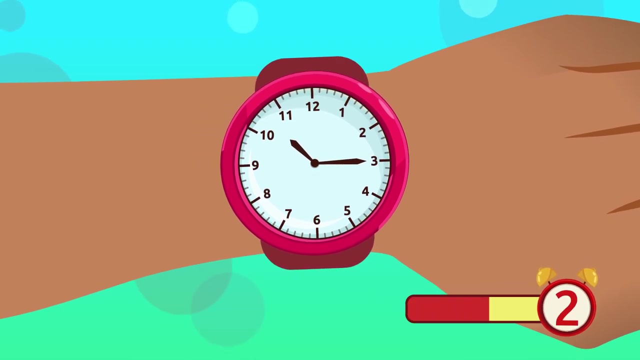 For example, it's a quarter after 5.. It's a quarter after 6.. It's a quarter after 7.. And it's a quarter after 8.. How about you give it a try? What time is it? It's a quarter after 10.. 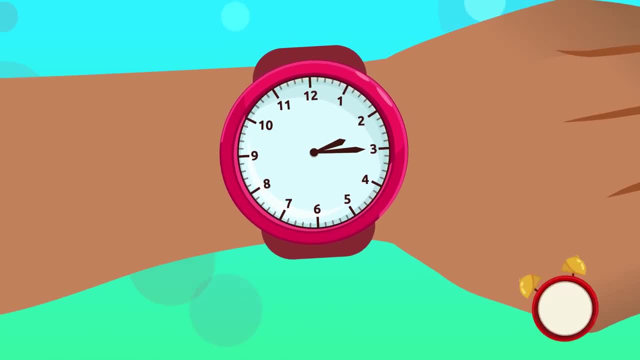 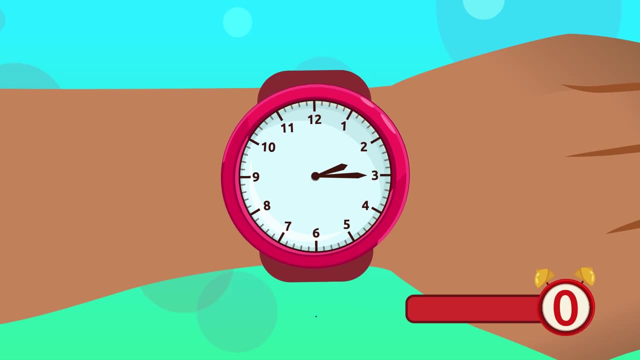 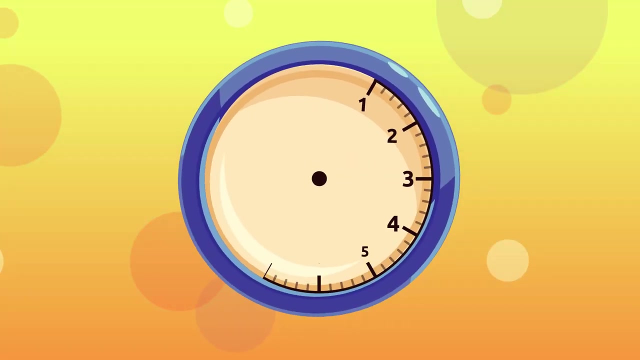 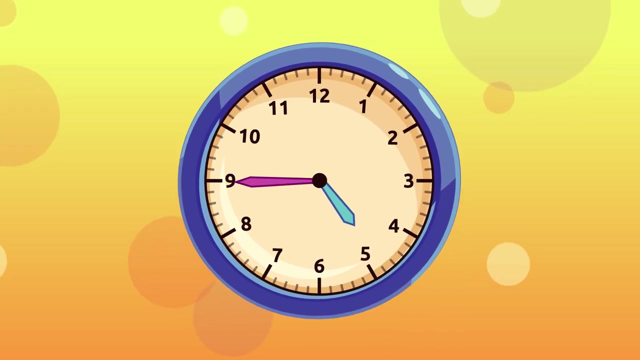 Very good. How about now? What time is it? It's a quarter after 2.. Good job. Finally, let's see what happens if we move the minute hand to the number 9.. How would you say? this time, As you can see, it is moved from the number 12 to the number 9.. 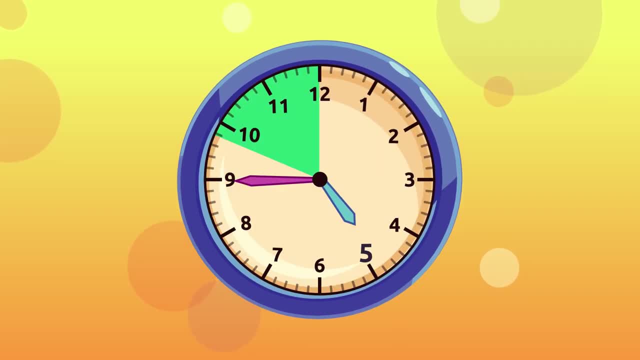 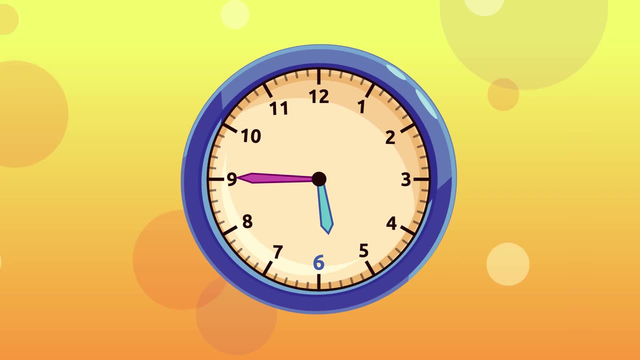 There is only a quarter left until it completes the hour. What if the minute hand is on the number 9?? Look at this example: The hour hand is closer to the 6, and the minute hand is on the 9.. That means it's a quarter of an hour left until it completes the hour. 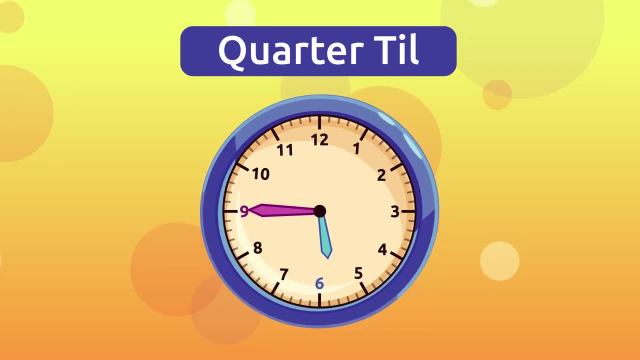 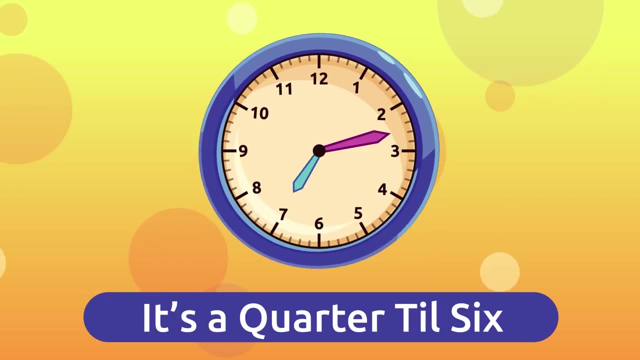 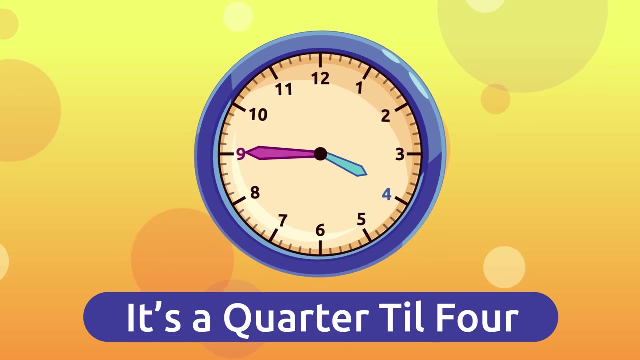 It is 1 quarter of an hour left until it completes the hour. So we say it is 1 quarter till six. Easy right, It is 1 quarter till 3.. It's a quarter till 4.. It is a quarter till 5..